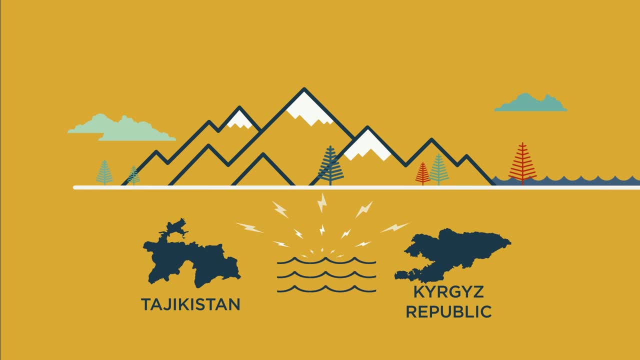 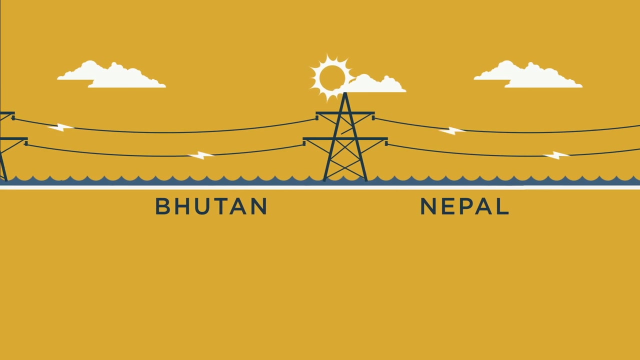 Countries such as Tajikistan and Kyrgyz Republic have hydro resources well in excess of their domestic needs, and Pakistan and India could offer them major import markets. Regional cooperation can also help tap natural complementarities, For example, when Bhutan and Nepal rivers are full of water in the summer. 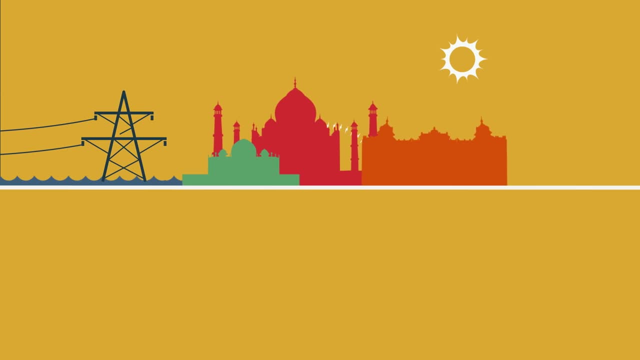 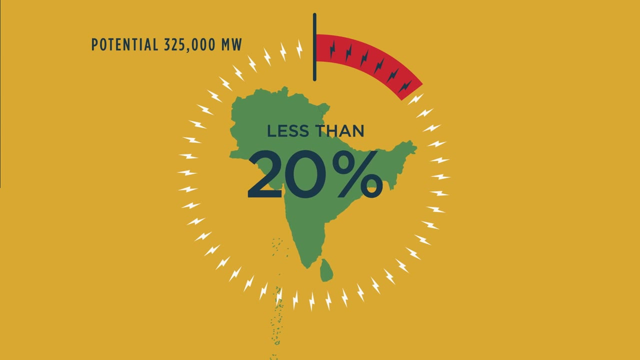 with vast hydropower generation potential. India and Bangladesh have the biggest demand for electricity to cope with the summer heat. Still, less than 20% of South Asia's hydropower potential is developed and energy sharing remains minimal By developing its hydropotential. 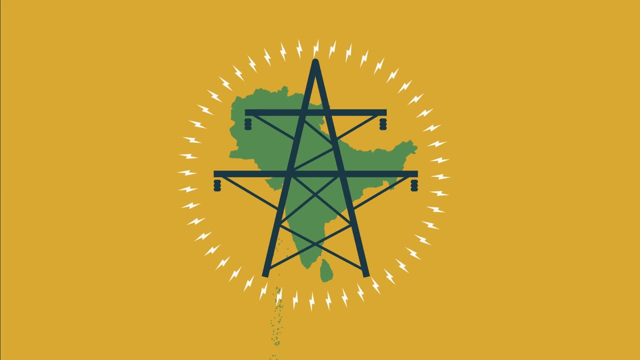 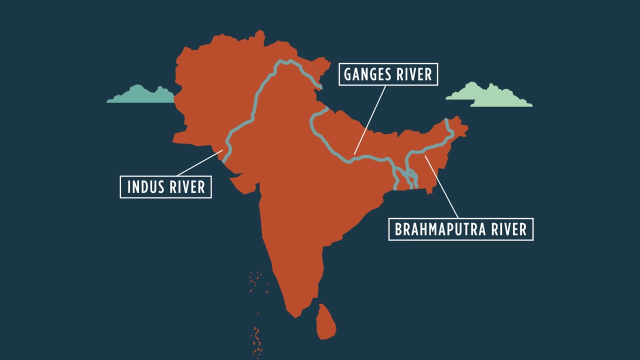 building cross-border transmission lines and eventually emerging into a regional energy market, electricity can reach thousands of energy-starved businesses and millions of people still living in the dark. Sharing water, The great rivers of South Asia offer more than just energy potential: They support life and supply resources. 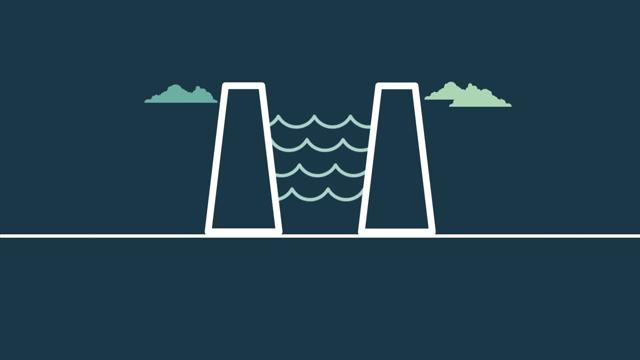 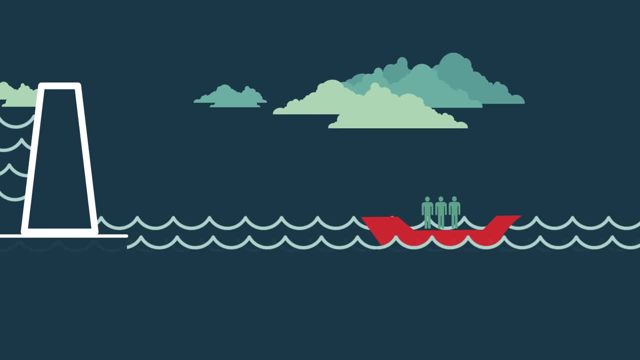 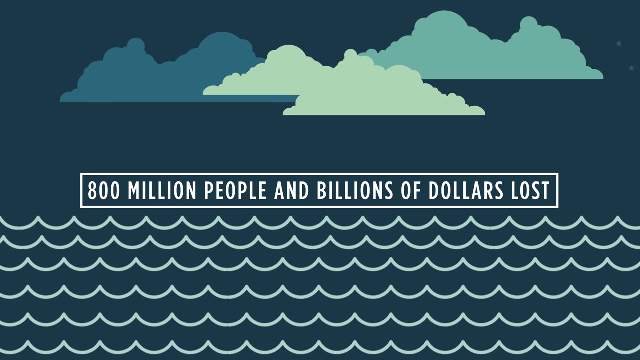 However, conflicting demands on these waters cause tension, distrust and little or no cooperation between countries, And the risks from natural disasters and climate change continue to grow. In the past two decades, natural disasters have affected over 800 million people and cost billions of dollars. 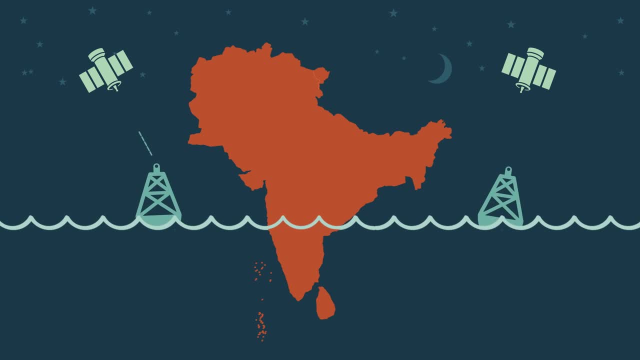 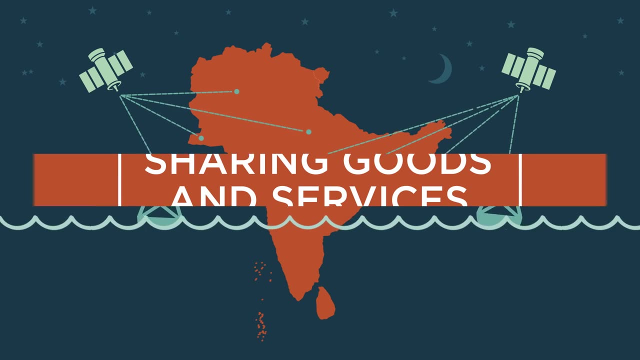 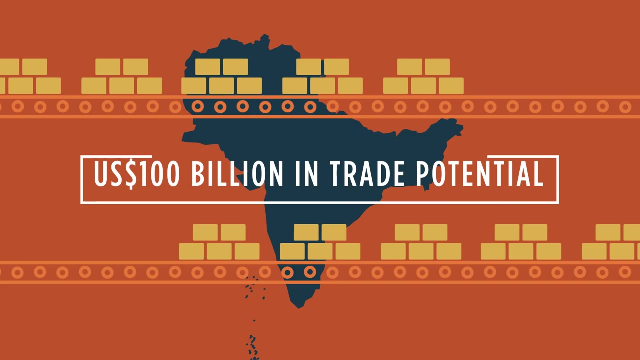 With cross-border cooperation on water and river basins, flood forecasting and early warning systems, lives and resources can be saved. Sharing goods and services Trade among the countries of South Asia could increase economic growth enormously. Yet South Asia's intra-regional trade is the lowest in the world. 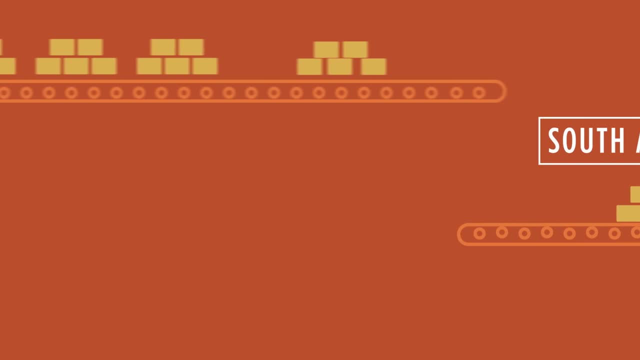 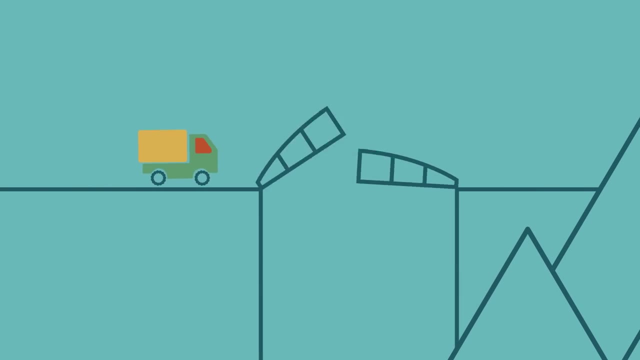 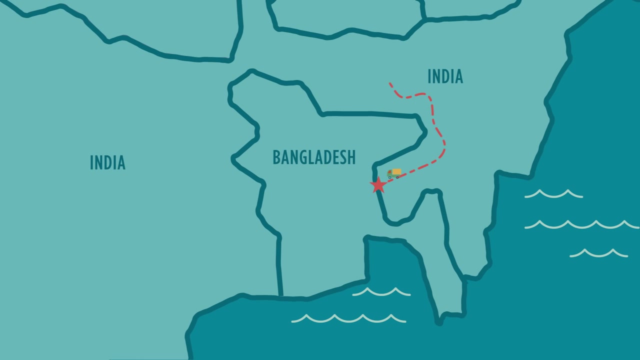 making up less than 5% of total trade. Landlocked countries and sub-regions are affected the most, since they depend on their neighbors for access to the sea and global markets. Goods are often moved through circuitous routes, sometimes traveling up to eight times the distance to reach their destination. 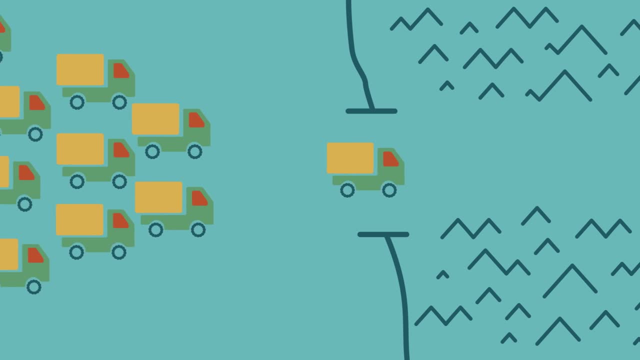 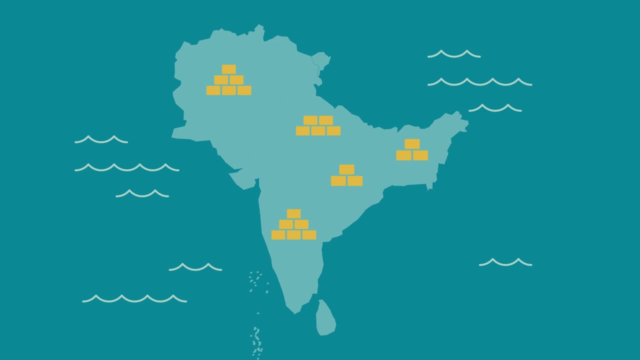 And border crossings are often so heavily congested that they can take days to cross. As a result, it costs more to trade within South Asia than with countries outside South Asia. For example, despite being geographic neighbors, the trade cost between India and Pakistan is 20% more.